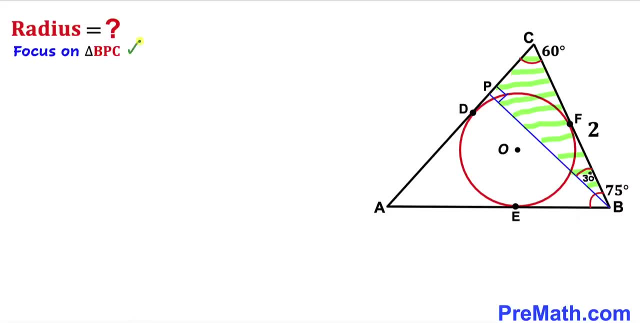 And now let's focus on this right triangle BPC, And now we can see that this is our 30,, 60,, 90 degrees. So therefore, this is our 30 degrees special triangle, And here I have copied down this triangle BPC over here And we can see that this is our smallest leg, since this is opposite to our this smallest angle, 30 degrees. 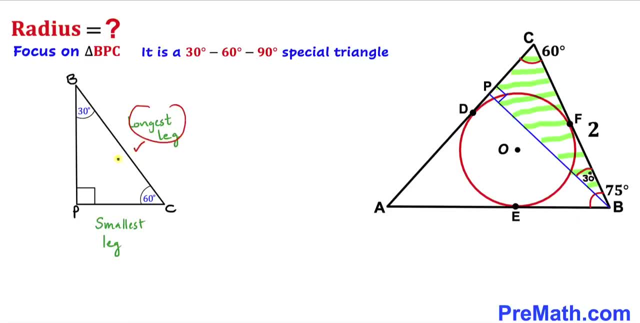 Whereas this leg is our longest leg, since this is opposite to this largest angle- 90 degrees. So in such kind of 30,, 60,, 90 degree triangle, this longest leg is always twice the smallest leg. If the smallest leg is always twice the largest leg, then we have to say that this is our 30,, 60,, 90 degrees. 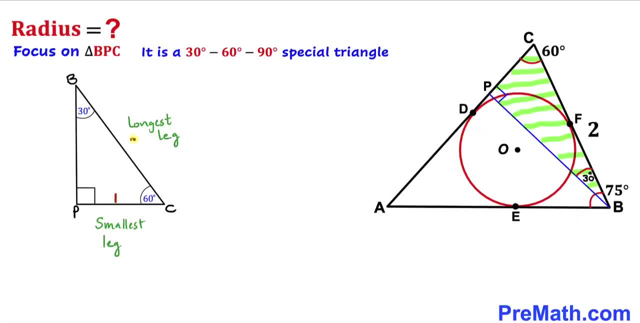 is one unit, then this longest leg is going to be two. and now we can see, in this triangle, our largest side is two units. so therefore, our this smallest leg is going to be one unit. that means bc is going to be one. so therefore, in this right triangle, bpc, our this side length is two, this is one. so let's. 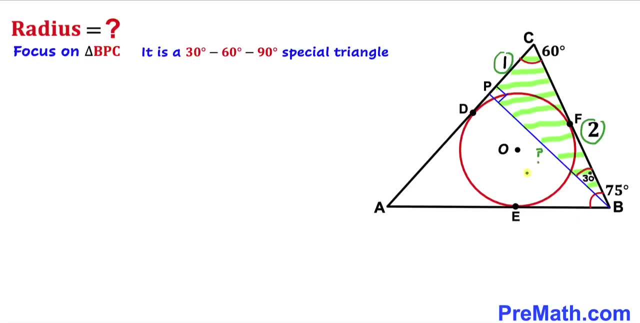 go ahead and calculate this unknown side length, bp. so therefore, we are going to use the pythagorean theorem. and here's our pythagorean theorem: a square plus b square equal to c square. let me go ahead and call this longest leg as our side c. let me label this unknown side as: 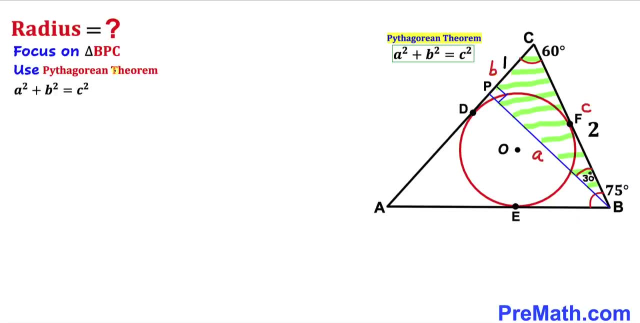 lower case a and this side lower case b. so let's go ahead and fill in the blanks in this pythagorean formula: a square plus b, in our case, is one whole square and c is 2 whole square. Let's go ahead and subtract 1 from both sides. This is gone, So a square turns. 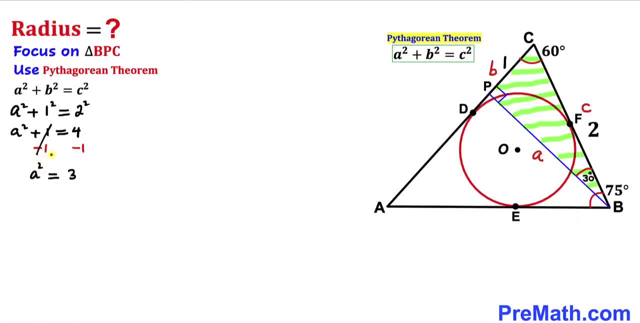 out to be 3.. Let's go ahead and undo this square by taking square root on both sides. So therefore, a value turns out to be square root of 3.. So therefore, our this unknown side a, which is the same as this bp length, turns out to be square root of 3 units. And now let's make an observation. We 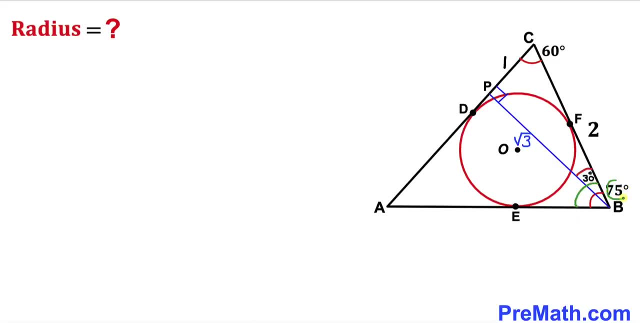 can see that this whole angle is 75 degrees and this angle is 30 degrees, So therefore, this angle has got to be 75 minus 30 is going to give us 45 degrees. And here's our next step. Let's focus on 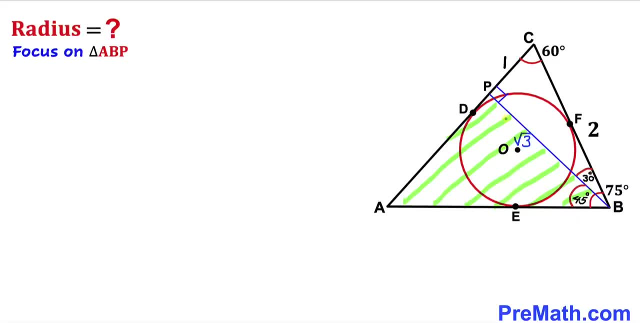 this triangle abp. We know that this angle is 90 degrees. This angle is 45 degrees. So therefore, this angle has got to be 45 degrees. And now we can see in this triangle: this angle is 45 degrees, This angle is 45. 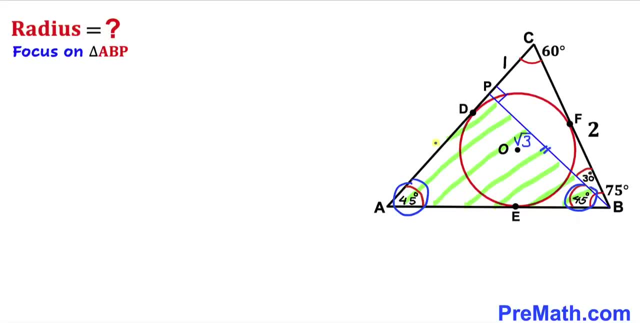 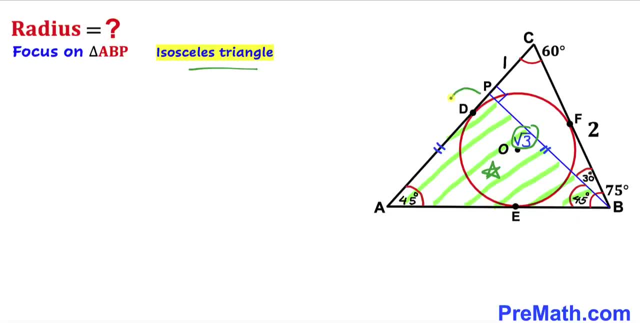 If this side length is square root of 3, then this AP length is going to be square root of 3 as well. So therefore, this whole side length AC is going to be 1 plus square root of 3.. So I can write 1 plus square root of 3.. 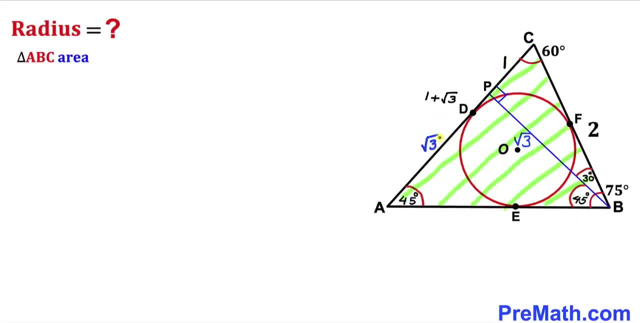 And here's our next step, Let's focus on this triangle ABC. We are going to calculate the area of this triangle ABC now, And now let's recall the area of a triangle. formula: Area equals to 1 half times base times height. 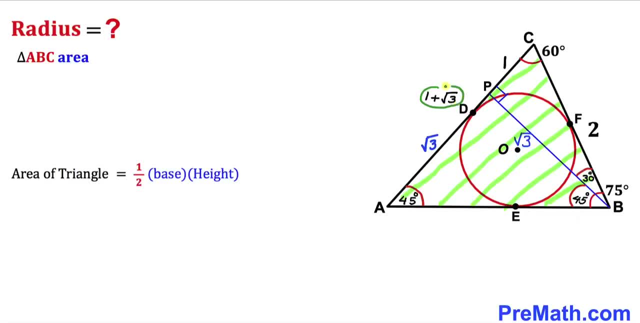 And in our case, this 1 plus square root of 3 is our base And this square root of 3 is our height of this triangle ABC. So, therefore, the area of this triangle ABC is going to be 1 half times our base is 1 plus square root of 3. 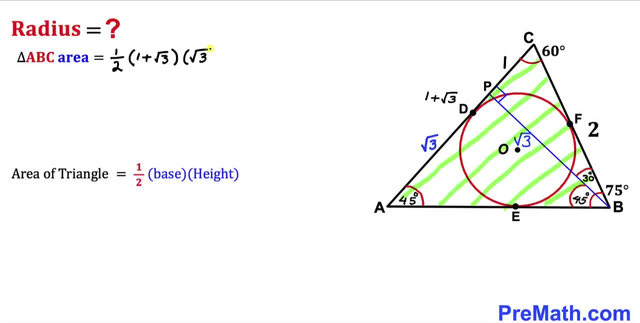 times our height is square root of 3.. Now let's go ahead and distribute this square root of 3.. 1 times square root of 3 is going to be square root of 3 plus square root of 3 times square root of 3. 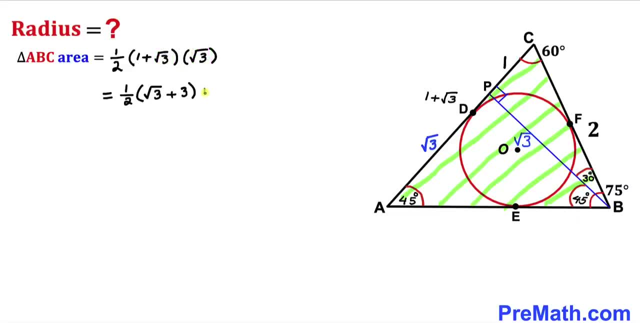 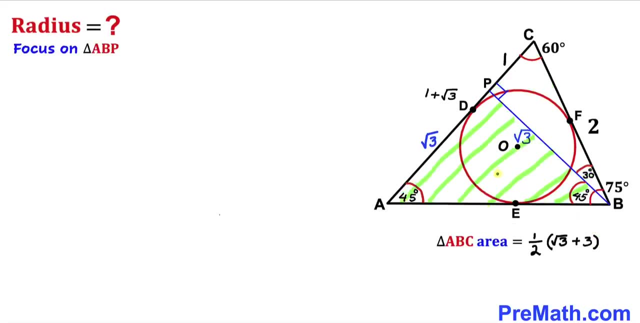 is going to give us simply 3,, as you can see in this next step. So, therefore, we figured out the area of the triangle ABC And now let's focus once again on this right triangle ABP, And we are going to use the Pythagorean theorem to calculate this unknown side length ABC. 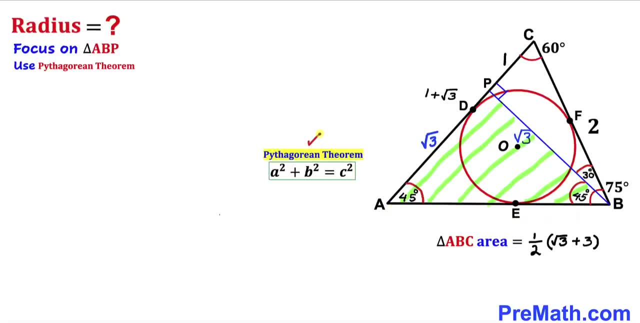 AB of this triangle. And here's our Pythagorean theorem. once again, Let me go ahead and call this longest leg as our side C. I'm going to call this side lowercase a and this lowercase b. So let's go ahead and fill in the blanks in this Pythagorean formula. 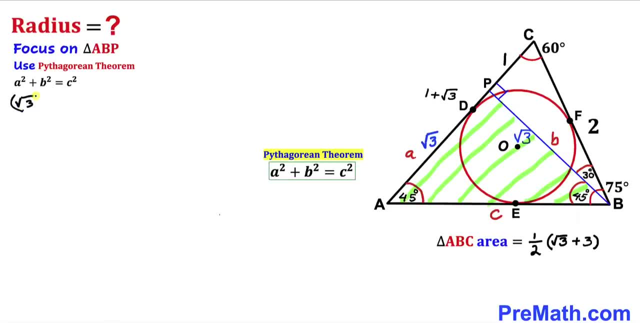 A in our case, is square root of 3 whole square, plus. likewise is going to be square root of 3 whole square equal to C square, And if we simplify this one, We're going to get C square equal to 6.. Go ahead and undo this square by taking the square root on both sides. 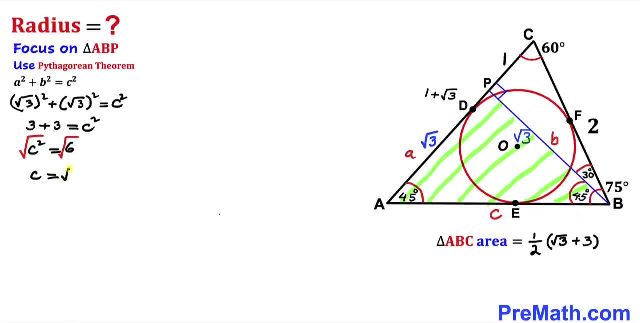 So, therefore, C turns out to be square root of 6.. So, therefore, our this side length, AB, turns out to be square root of 6 units. Here, in this next step, I have connected this center O with these points of tangency. 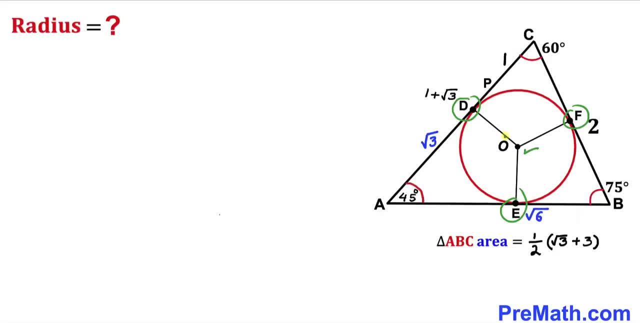 E, F and R D, as you can see over here. And now we can see that these are our radii. Let me label this radius as lowercase r, Lowercase r and lowercase r as well. And now let's recall the circular theorem. 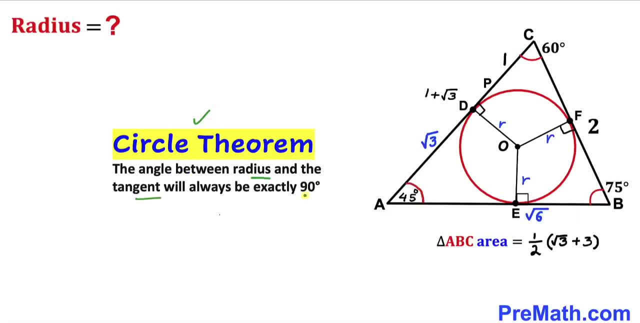 According to this theorem, the angle between the radius and the tangent will always be 90 degrees. And no wonder all these angles are going to be 90 degrees, Since these are our radii and these are our tangent lines. And now, in this next step, I have connected this center O with these vertices A, B and C. 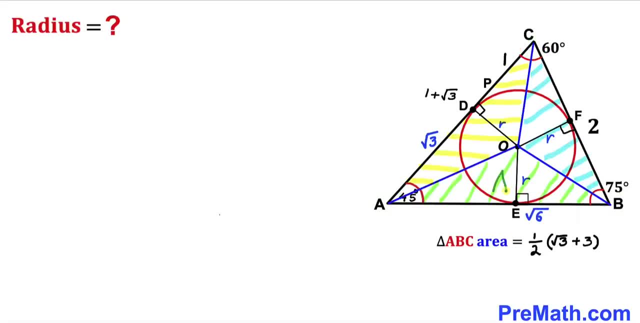 And, as a result, we got these three triangles AOB, This other triangle AOC and this triangle BOC. And now let's make an observation. We can see the area of this whole triangle ABC is going to be equal to the sum of these individual area of triangles. 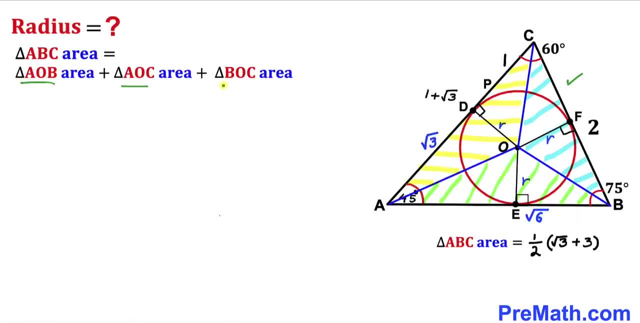 We can see the area of this whole triangle. ABC is going to be equal to the sum of these individual area of triangles AOB, AOC and BOC, And we already figured out our ABC triangle area. So now our task is to calculate the area of these individual triangles: AOB, AOC and BOC. 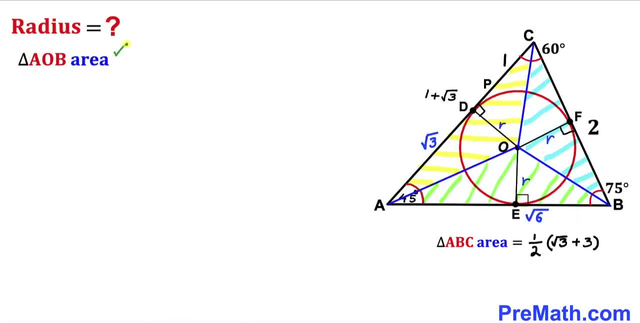 And now let's go ahead and calculate the area of this triangle, AOB, And let's recall the area of a triangle. formula: Area equals to a half time base times height. Area equals to a half time base times height. In our case, our base is square root of 6 and our height is radius r. 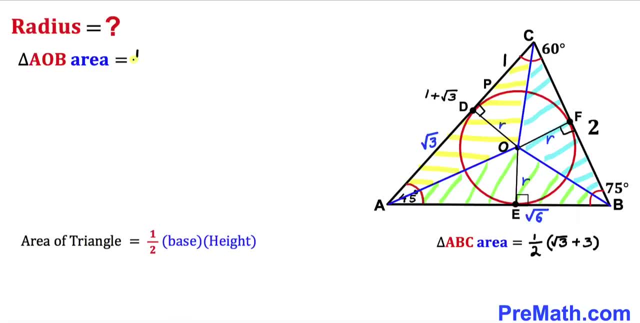 So therefore, the area of this triangle AOB is going to be a half times. our base is square root of 6 times lowercase r And we can write this one as 1 divided by 2 times r, times square root of 6.. 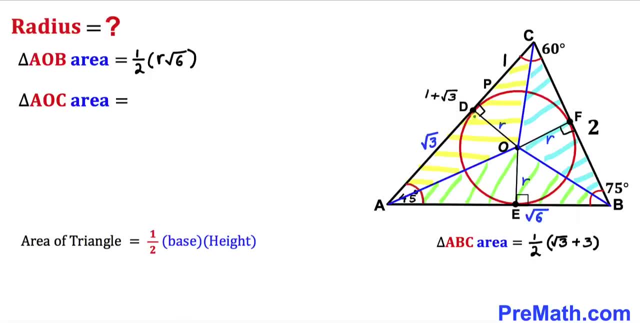 And now let's go ahead and calculate the area of this other triangle, AOC, whose base is 1 plus square root of 3.. And we can write this one as 1 divided by 2 times r times square root of 6.. And height is radius r. 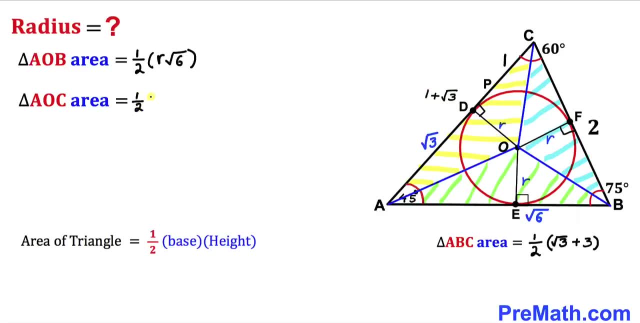 So, therefore, we can write 1 divided by 2 times 1, plus square root of 3 times lowercase r. And finally, let's go ahead and calculate the area of this triangle, BOC, whose base is 2 and height is radius r. 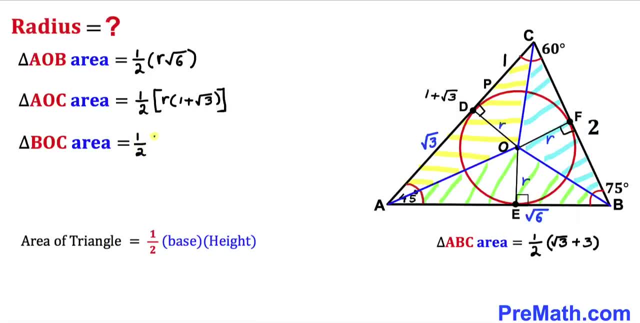 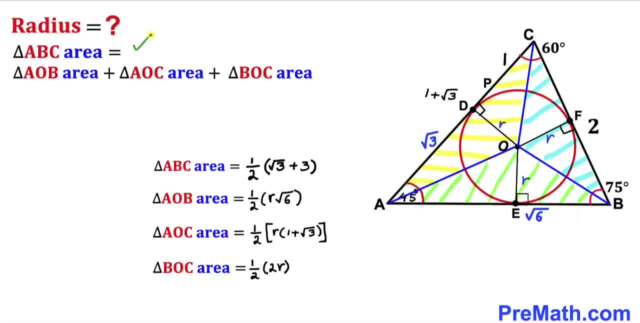 So, therefore, the area is going to be a half times, 2 times lowercase r. And here is our next step. We are going to fill in the blanks in this equation since we figured out all these individual areas. As you can see, in this next step I have replaced this triangle ABC area over here on the left hand side. 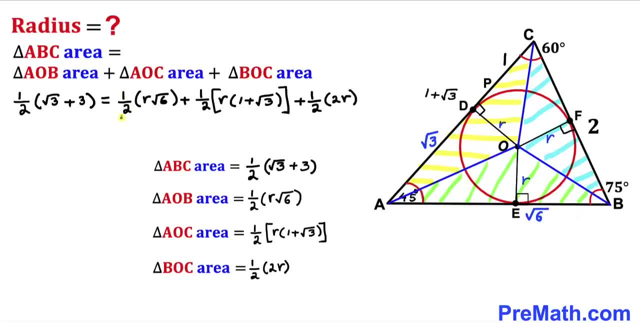 equals to, on the right hand side, the area of this triangle AOB, the area of this triangle AOC and, finally, area of this triangle BOC. over here And now, let's go ahead and calculate the area of this triangle AOB. Now let's make an observation. 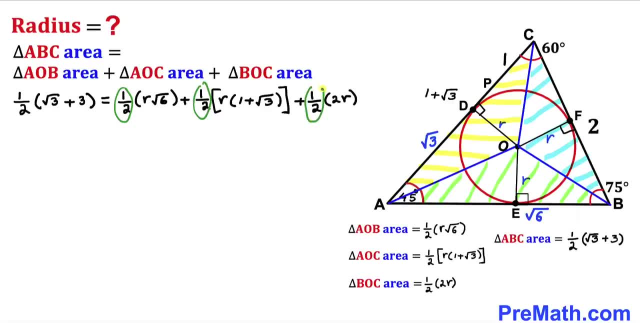 We can see that 1 divided by 2 is in common on the right hand side and this radius r is in common as well. So therefore I have factored out 1 divided by 2 times r outside, and the rest is inside this bracket. 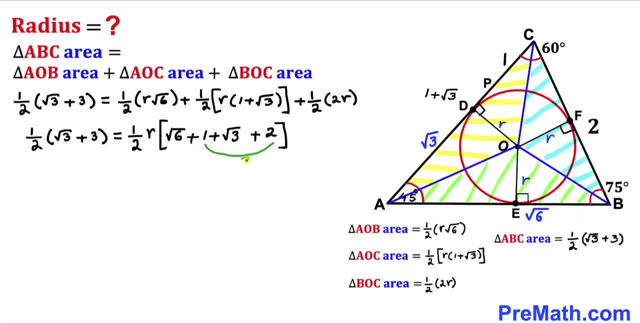 And if we combine these like terms, 1 plus 2 is going to give us 3.. As you can see in this next step, I have combined these like terms over here And now we can see this: 1 divided by 2 and 1 divided by 2, they cancel each other out. 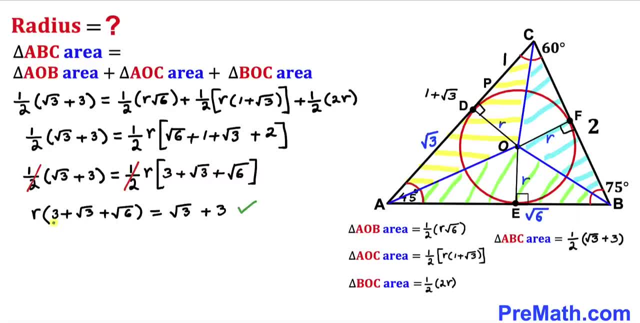 So therefore, we are ended up with r times 3 plus square root of 3 plus square root of 6 equals to square root of 3 plus 3 on the right hand side. Now, in this next step, I have divided both sides by this: 3 plus square root of 3 plus square root of 6, as you can see. 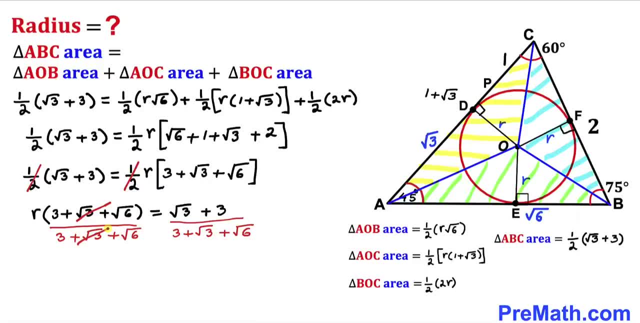 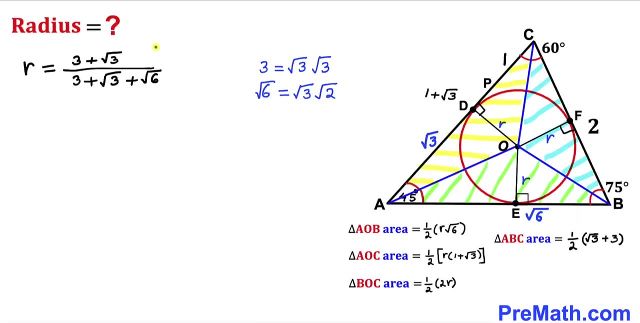 And we can see that this cancels out with this. So that's our radius. r turns out to be 3 plus square root of 3, divided by 3 plus square root of 3 plus square root of 6.. And now let me go ahead and manipulate this rational equation. 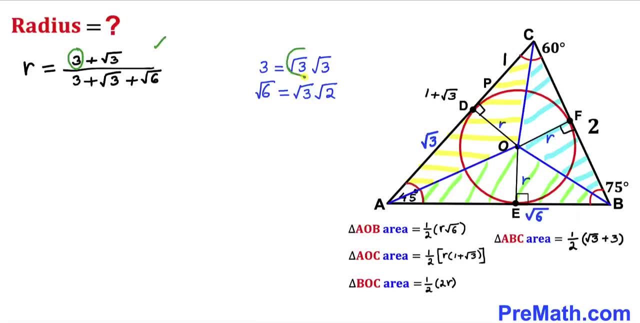 I'm going to replace this 3 by 3 square root times square root of 3.. And likewise, this square root of 6 at the denominator could be written as square root of 3 times square root of 2.. As you can see, in this next step, I have replaced this 3 by square root of 3 times square root of 3.. 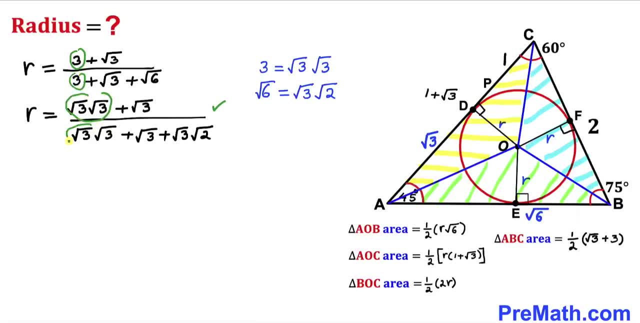 Likewise at the denominator, this 3 by same thing, And over here square root of 6 by square root of 3 times square root of 2.. And now we can see square root of 3 is in common at the numerator. 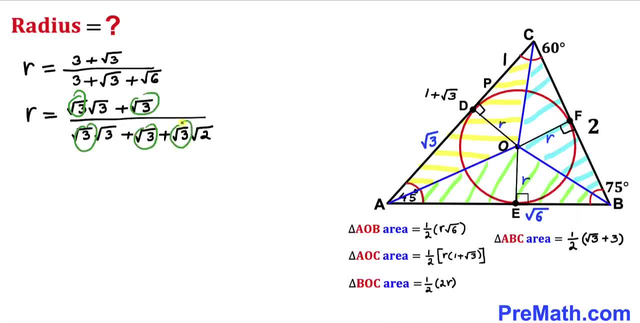 And likewise square root of 3 is in common at the denominator as well. As you can see, in this next step I have factored these square root of 3 outside on both numerator and denominator, And now we can see this square root of 3 and square root of 3, they are gone. 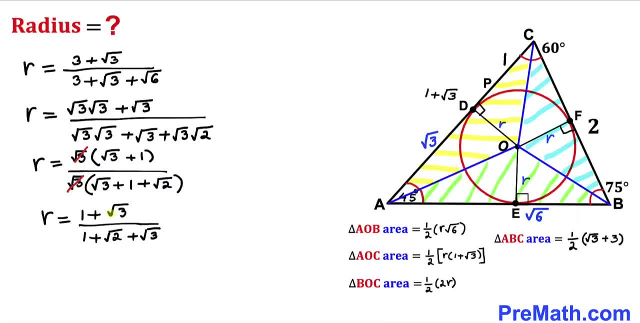 So therefore we are ended up with: r equals to 1 plus square root of 3, divided by 1 plus square root of 2 plus square root of 3.. And now let's go ahead and rationalize the denominator. So I'm going to multiply and divide by 1 plus square root of 2. 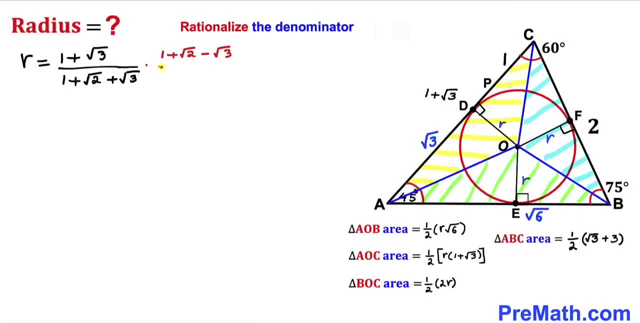 minus square root of 3.. Likewise, I'm going to divide this one as well. And now let's go ahead and multiply these numbers on the top and these one at the bottom as well. Now, let's go ahead and distribute these ones at the top first. 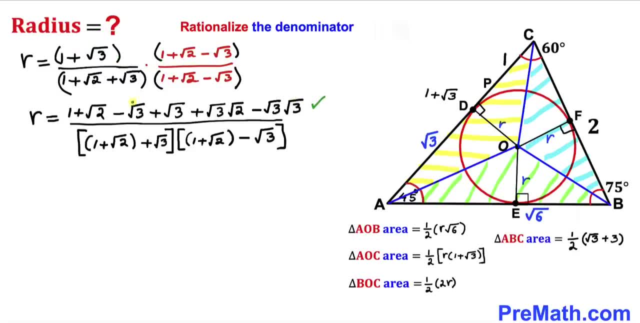 As you can see in this next step I took care of this numerator And at the denominator I have chunked these ones. I wrote down 1 plus square root of 2 over here and then square root of 3 over here. 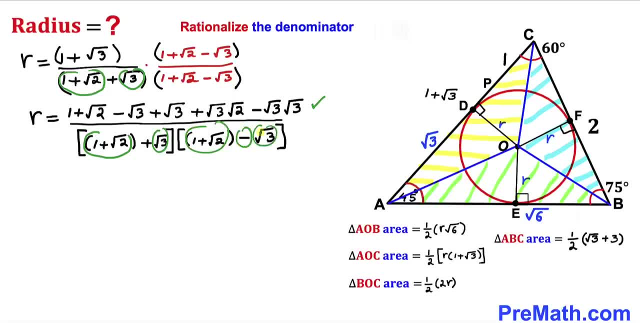 Likewise this one with a negative sign in between. And now we can see this positive square root of 3 and negative square root of 3, they are gone And I'm going to replace this square root of 3 times square root of 3 as 3.. 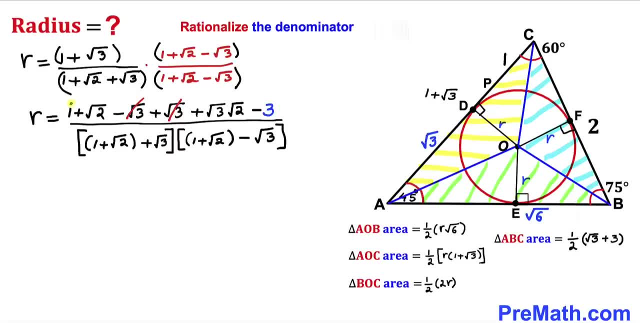 As you can see over here. And now let's combine these two numbers: 1 minus 3.. That is going to give us negative root of 2.. As you can see over here on the numerator. And now let's recall this famous identity: a plus b times a minus b could be written. 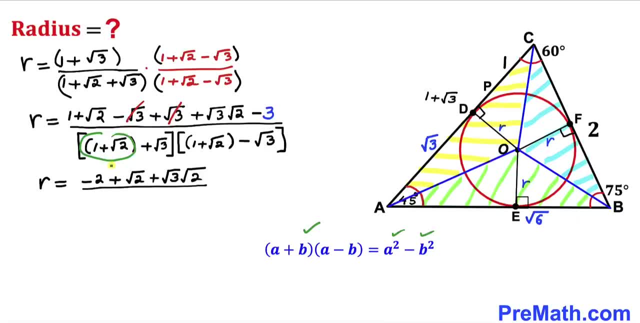 as a square minus b square. If I call this our a and this our b, likewise this our a and this our b, then the denominator is going to become 1 plus square root of 2 whole square minus square root of 3 whole square. 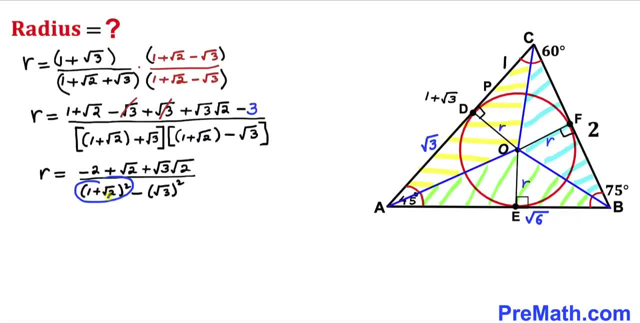 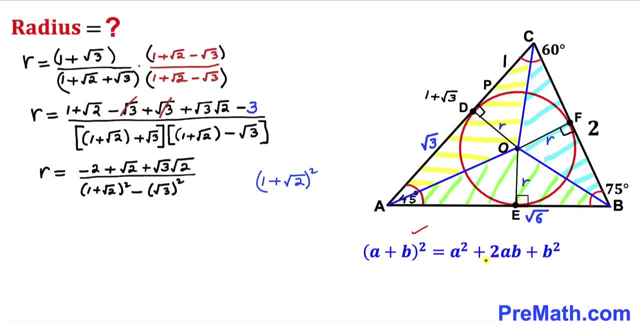 and now let's focus on this part 1 plus square root of 2 whole square. and here I have copied it down. and now let's recall this identity: a plus b whole square could be written as a square plus 2, ab plus b square. we are going to apply it over here and if we simplify, this turns out to be: 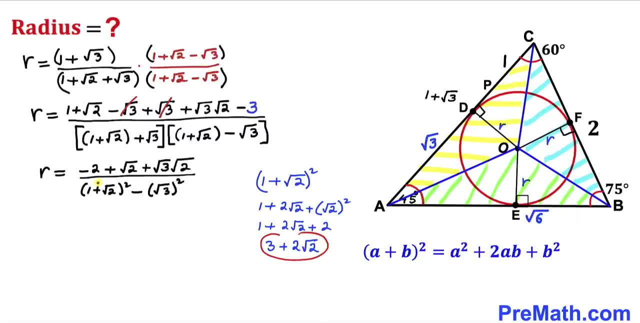 3 plus 2 times square root 2, so therefore, I'm going to replace this part by this and this square root of 3 whole square could be written as 3, as you can see in this next step, I have replaced this one by this, as you can see over here, and this square root of 3 whole square turns out: 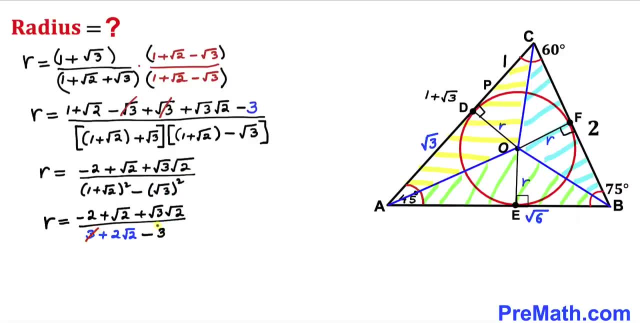 to be simply 3, and now we can see at the denominator 3 and minus 3, they cancel each other out. so therefore, at the denominator, we ended up with 2 times the square root of 2. now we are almost finished. let me go ahead and tweak this: 2: 2 could be written as square root of 2 times square root. 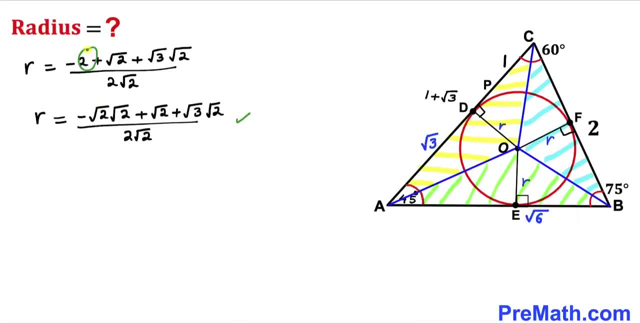 of 2. As you can see, in this next step I have replaced this 2 by square root of 2 times square root of 2.. And now we can see square root of 2 is in common at the numerator. So therefore we factored out square root of 2 outside. 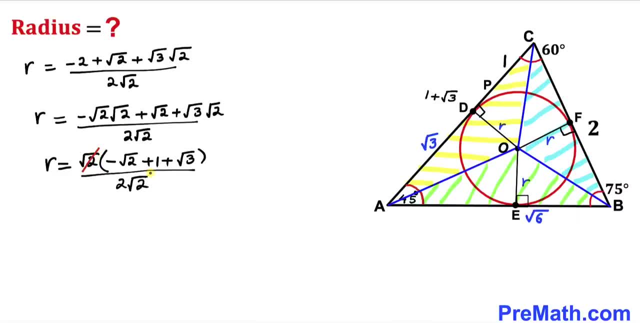 And now we can see the square root of 2 at the numerator and square root of 2 at the denominator. They cancel each other out. So therefore, finally, our radius r turns out to be 1 minus square root of 2 plus square root of 3 divided by 2..